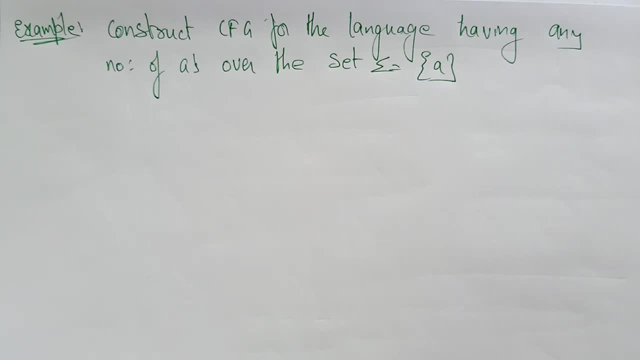 Hi students, welcome back. In the previous video I explained about what is a context-free grammar. That is a context-free grammar. It's a combination of the. it's defined as a four tuples: V T P S or N T P S. 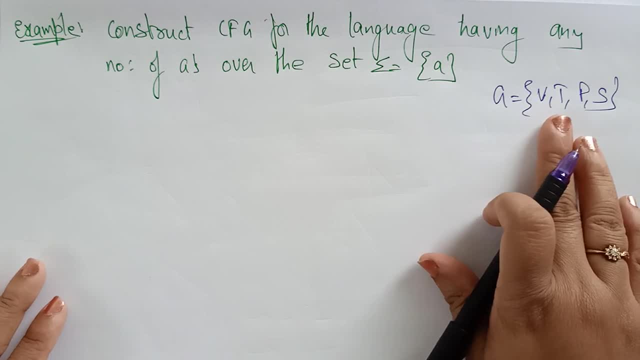 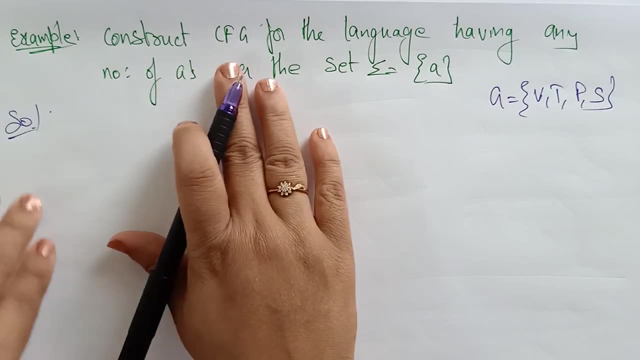 V is a set of non-terminals, T is a set of terminals and P is the production rules and S is a start symbol. So here they are asking the question: like we need to construct the context-free grammar. Okay, one context-free grammar we have to be generated. 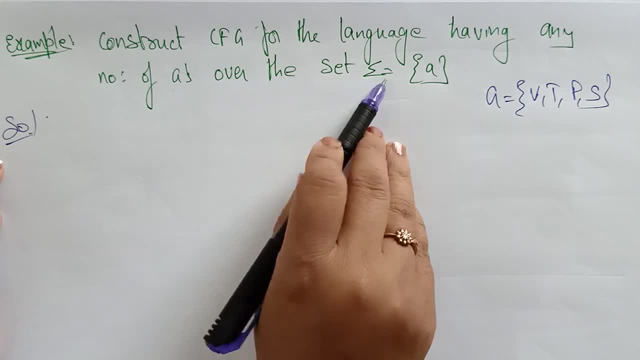 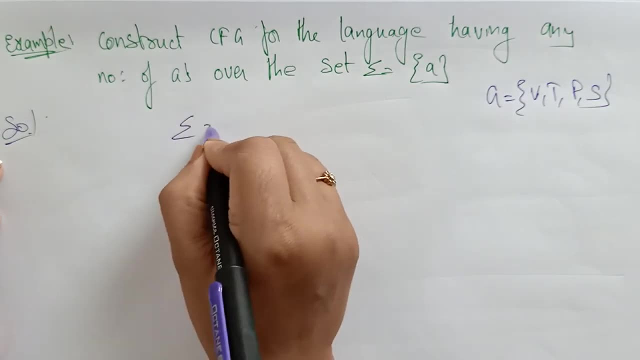 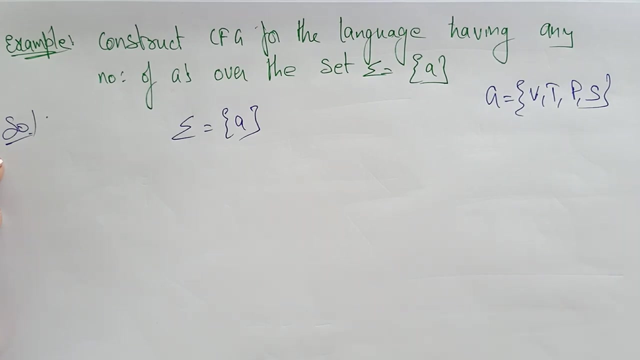 For the language. having a number of A's over the set means any number of A's. having any number of A's- Okay in the set. in the set, only the A. the input symbol is only the A- Okay, so it can be represented in any number of A's. 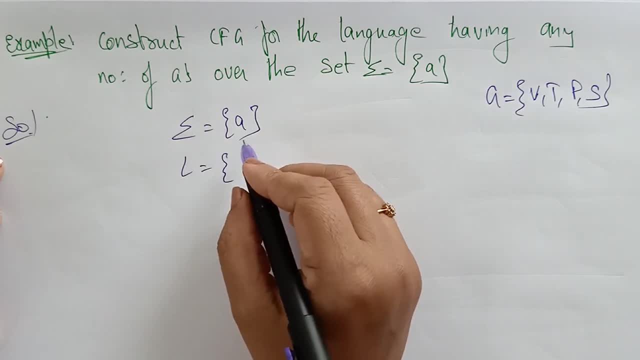 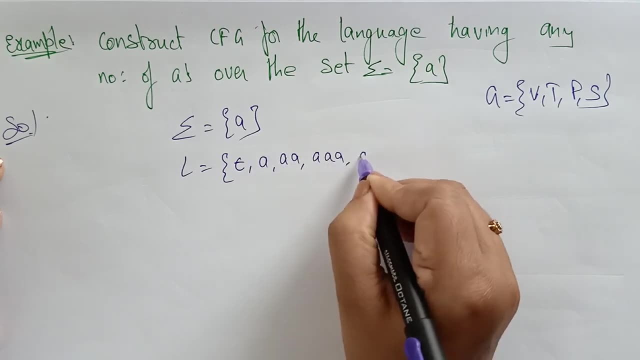 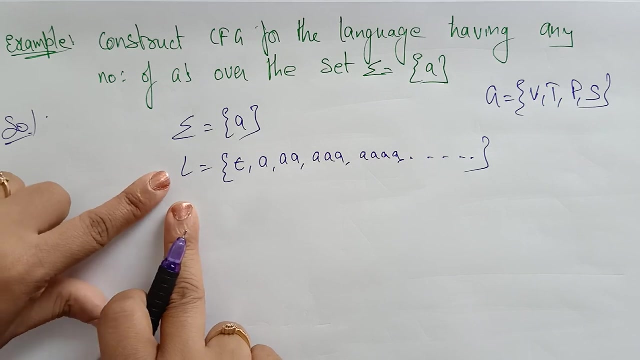 The language can be represented in any number of A's. That is including epsilon. you can include the empty string also: A, A, A, A. so like this, Any number of A's. Okay, by seeing the question, I have written like this: 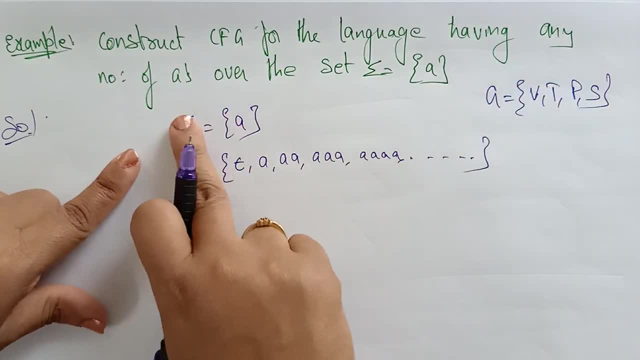 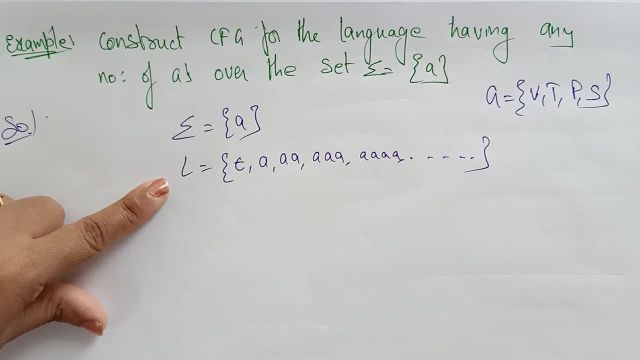 They are asking: construct context-free grammar for the language having any number of A's. So any number of A's means it may be 0 or 1,, 2,, 3,, 4, 5, any number of A's over the set. 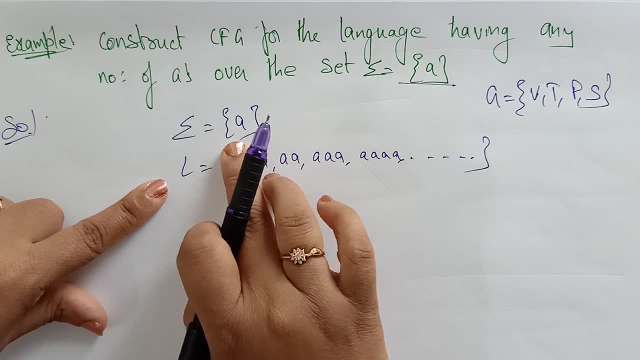 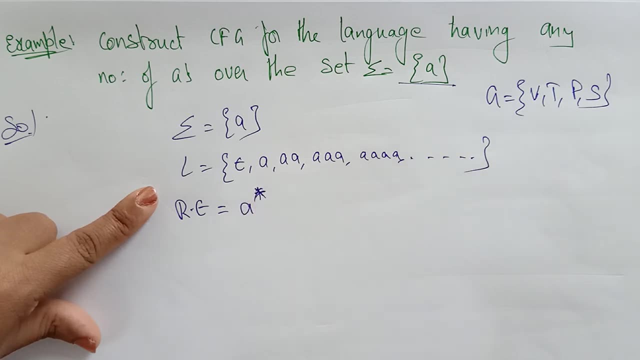 For this I need to construct the context-free grammar. How I can construct. So first let me write the regular expression for this grammar. The regular expression for this grammar is A star, Obviously, because A closure means A star, means it's a multiples of A. 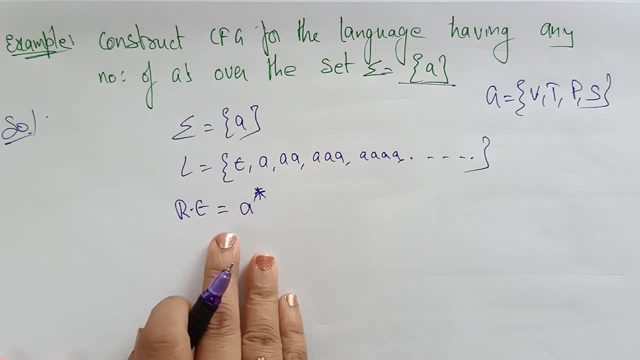 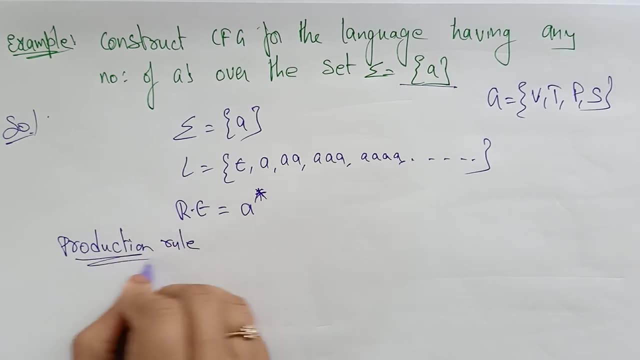 A, multiples of A, can be represented a regular expression like this. Now, coming to the production rules, First write the production rule for the context-free grammar. Okay, so the production rule for the regular expression. whatever the regular expression I got by seeing this regular expression, I am going to construct the production rule. 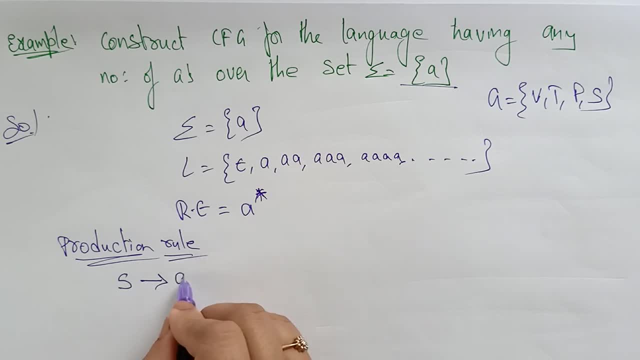 So I am taking the starting symbol as A S, Okay, and I take S as an epsilon. So I am calling this as rule 1 and this is as a rule 2.. Production 1, rule 1 and rule 2.. 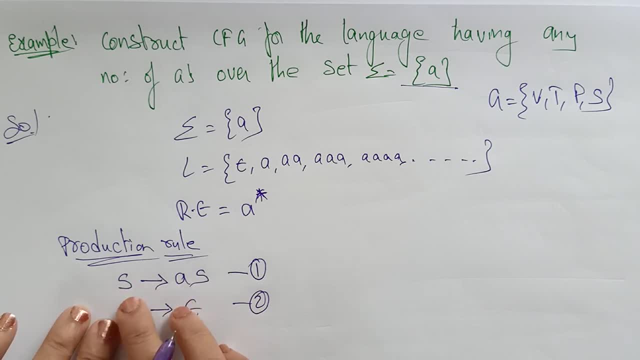 Means: S determines A means. I am replacing, in place of S, A S. Okay, so in place of S, I am replacing S with epsilon. Okay, so the right hand side, whatever it may be, that should be replaced to the left hand side. 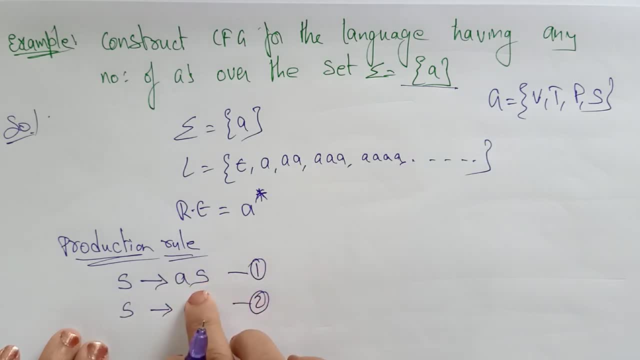 So in the place of S I can replace S with epsilon, So I can keep epsilon. A epsilon means you will get A only, So that is a regular expression that you are getting. So these are the production rules for the given regular expression. 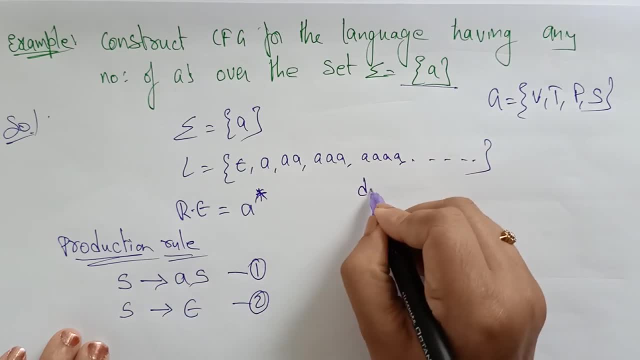 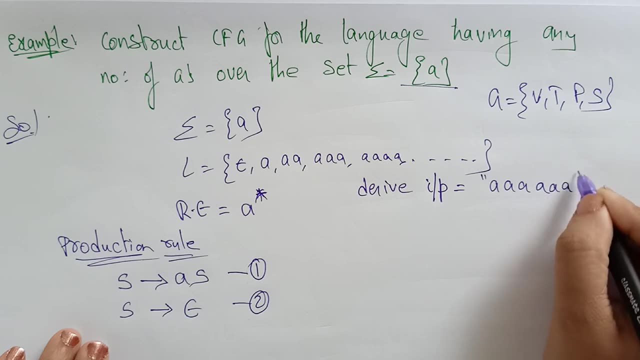 Now, if we want to derive a string, let me derive a string. That is the input. I am taking A, A, A, A A 6 As Okay. so this I need to be derived. The context-free grammar is set of non-terminals. 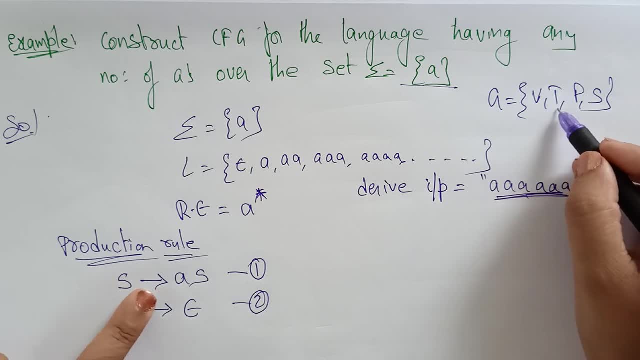 Here I have taken the non-terminals as S And the terminals. I am taking the terminals as a P And the production rules, or two production rules I am having, And S is a start symbol. Okay, so now I want to derive an input string. 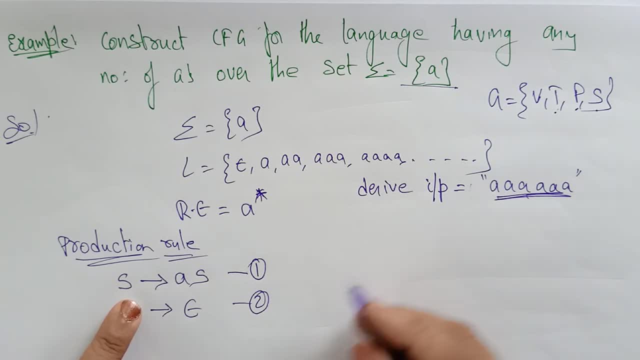 So this input string I need to be derived. Now we can start with the start symbol. So according to the rule, we have to start with the start symbol. So start with the S Now. replace S with the production rule. 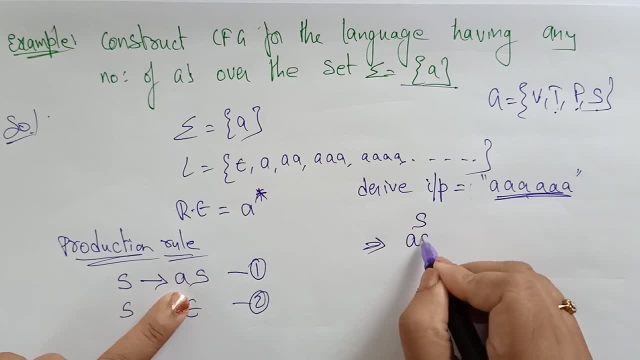 So, in place of S, I am going to write A S According to the rule. Okay, S is replaced with A S. Now again, I am replacing S with A S, Because I want to read this string. 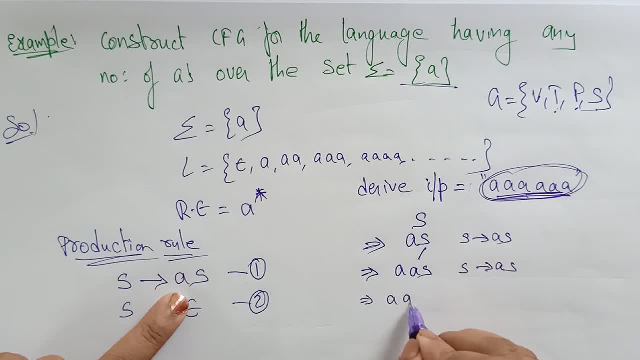 I want to derive this string Again. replaced S with A S. That is, S is replaced with A S. Until you get this string, Check while you are writing A A Again, replace S with A S. 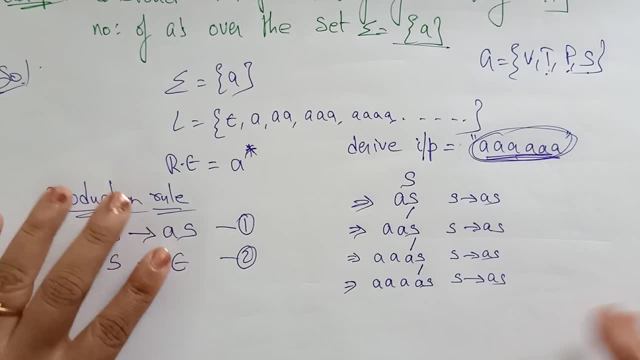 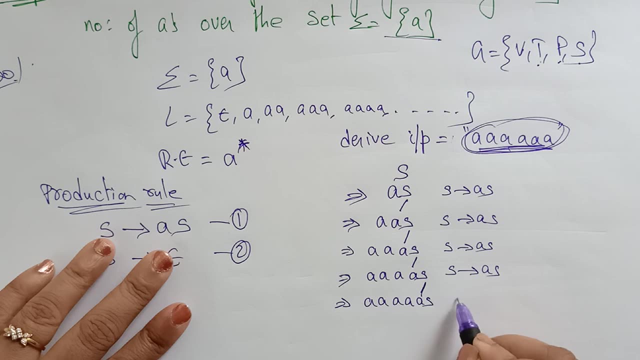 So I got 4.. I want to get the 6 A's here Again. replace S the production with A S, S replaced with A S. So I got here 5 A's: A, A, A, A. 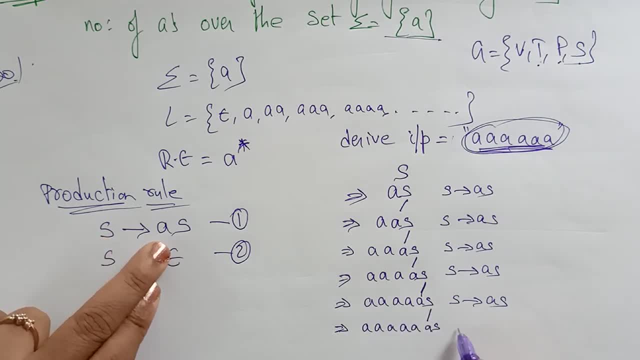 Again, I replaced S with A S. production, That is, S is replaced with A S. So how many A's? I got 6 A's, So I derived the input string. Now I am replacing S with epsilon.